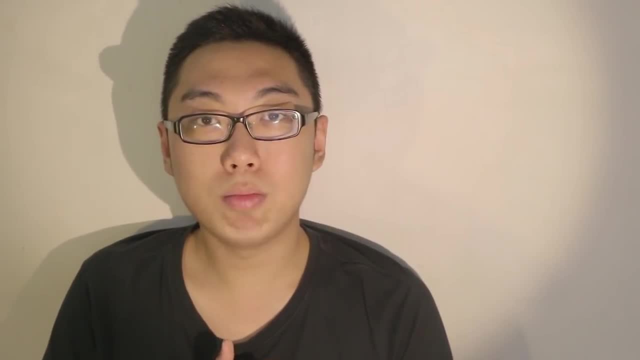 important things you need to know about this technique is that? well, it's only applicable in certain cases, Namely when you're working with an algorithm or a data structure that you know basically has multiple operations. Some of these operations are fast, some of them are. 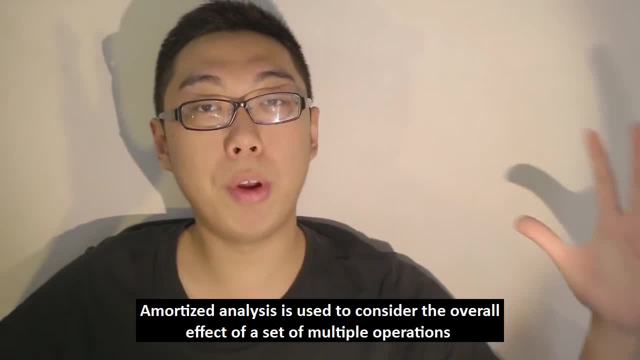 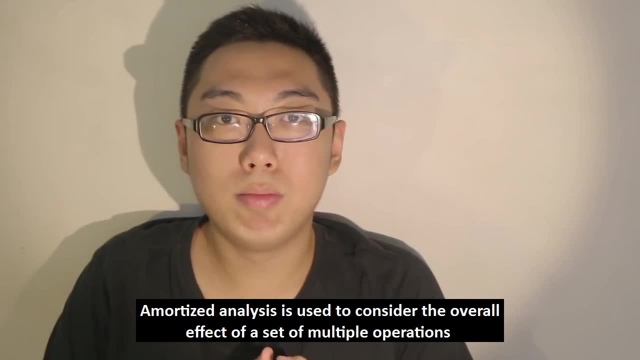 slow, And the idea is we want to look at a whole bunch of different types of operations At once and basically see what all these operations together tell us about. you know, a general sort of average operation on this data structure. There are actually three different. 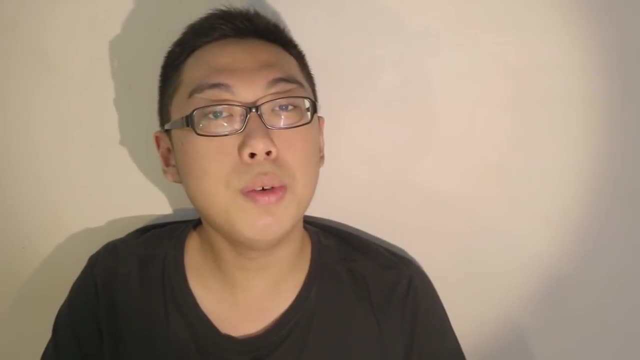 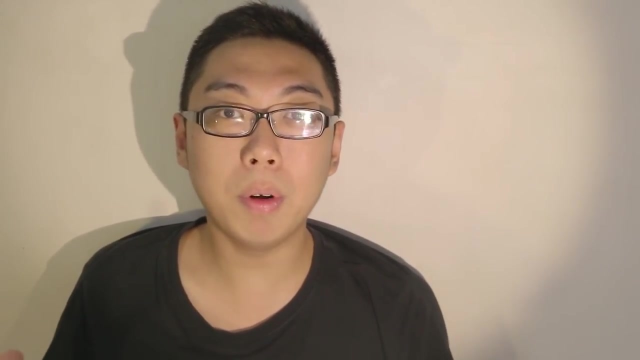 ways to perform amortized analysis, And today what we're going to do is we're going to scrape the surface of each. So we're going to briefly look at each, all in the context of the same example, And hopefully we'll paint, you know, a rough picture of how these techniques 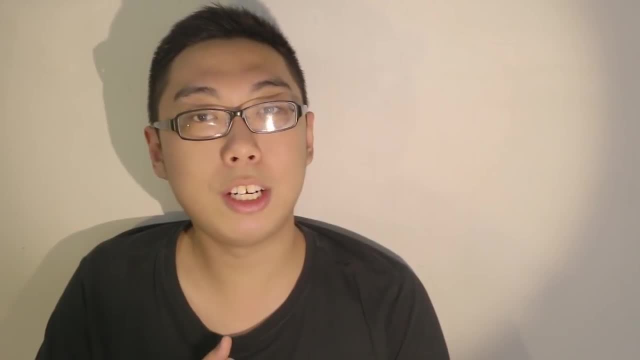 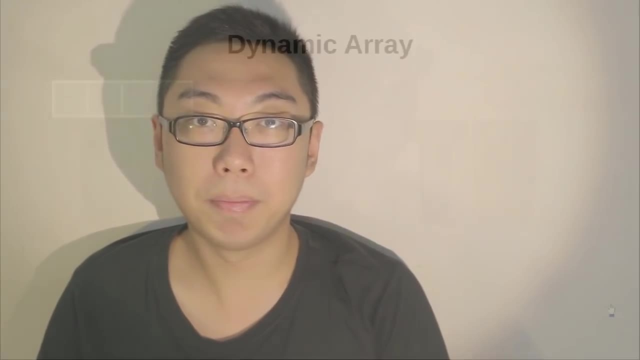 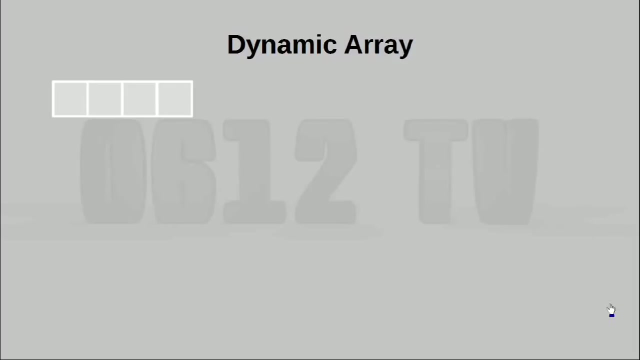 actually work. So yeah, without further ado, let's jump in first to the example and then to actually applying amortized analysis. One of the classic examples used to demonstrate amortized time complexity is a dynamic array data structure. Now here's how this works. Imagine we have a. 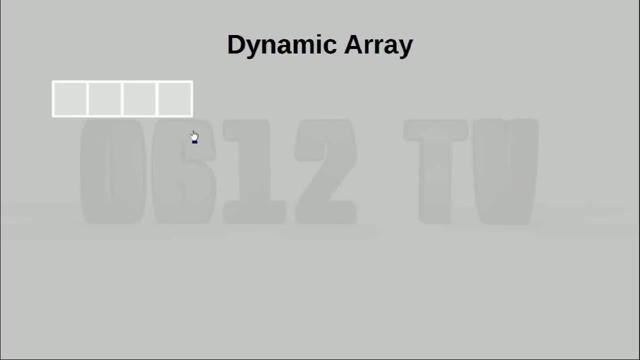 small array And the idea is that we want to insert an unknown number of items into this array. Of course, eventually the array gets full And the strategy used by this algorithm is that we are to create a new array that is double the size and to actually move everything across. This, of course, as you can, 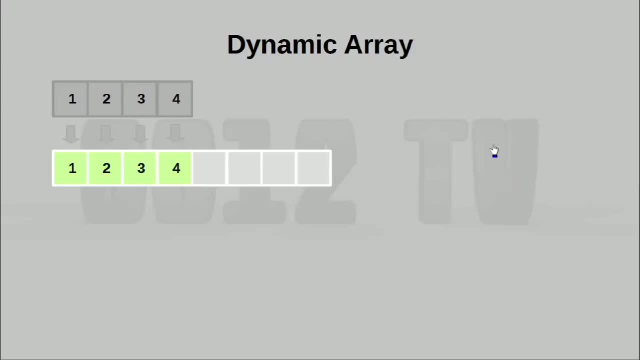 imagine is a slow process, which is why this is such a good candidate for discussing amortized time complexity. Of course, this doesn't just happen once. When we next fill up the array, we're going to have to do the same thing again. This step, of course, is also very expensive. 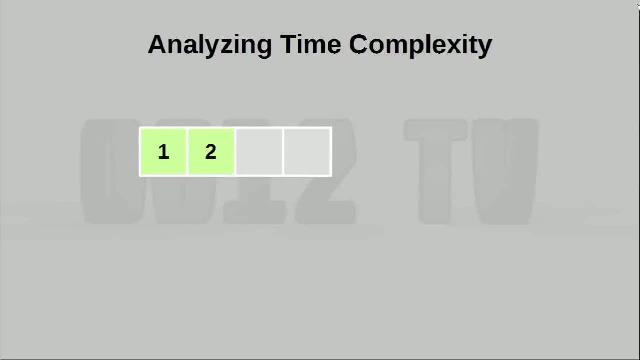 because we're copying even more items across. now Here's the deal. At face value, analyzing the time complexity of this gives us wildly inconclusive results. When I'm actually inserting an item that doesn't trigger an array expansion, well, that's basically instantaneous. That is a definite O1 operation. However, 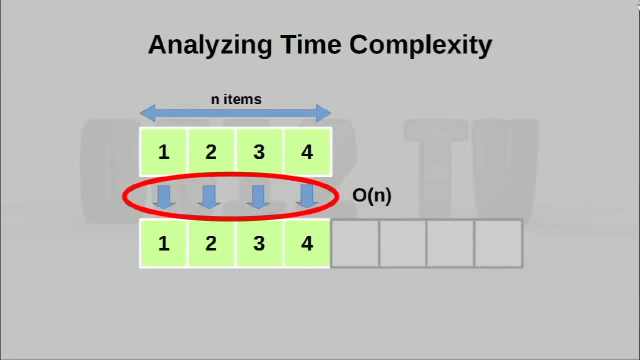 when I actually do trigger an array expansion. well, we're moving n items from one array to another, an ON step. So what really is the time complexity of a general operation on this data structure? That is the question that amortized time complexity tries to answer for us. 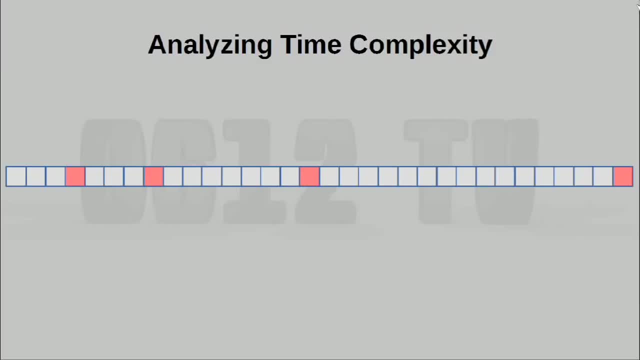 Now let's sort of actually step back and take a look at when these expansions happen. What that means is, for each one of these little gray boxes, we are doing one unit of work. However, when we encounter one of these red boxes, well, we're doing quite a lot of work. 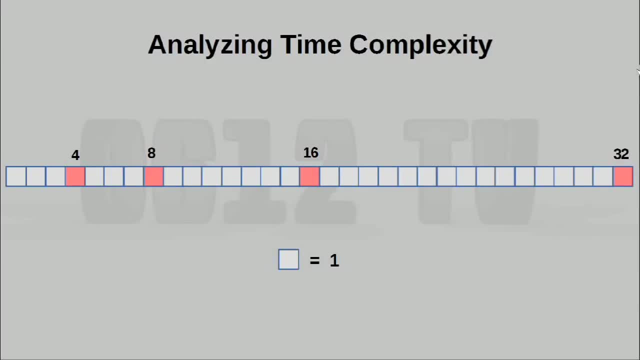 We're doing a lot of extra work on top of, you know, the normal insertion. We can also observe that every time this happens- it happens half as often but it does twice as much work- And perhaps intuitively you can sort of get the idea that these two things sort of cancel out and is somehow 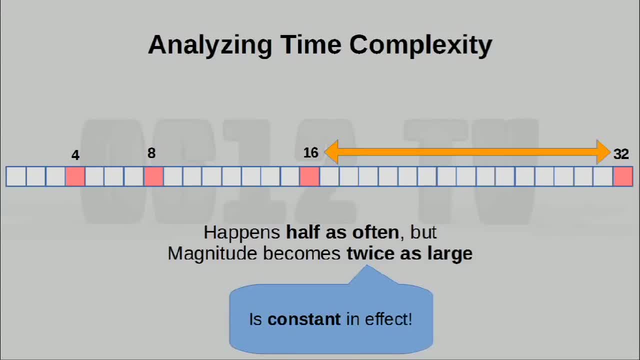 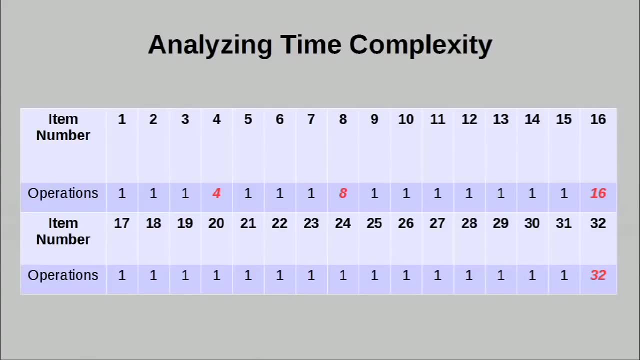 constant. in effect, By using amortized analysis, we can actually make this more concrete. This table is just a different way of showing you what we've just seen, which is, of course, the number of operations required for each step. Basically, what you're seeing here lends itself to one of the simplest ways of actually performing. 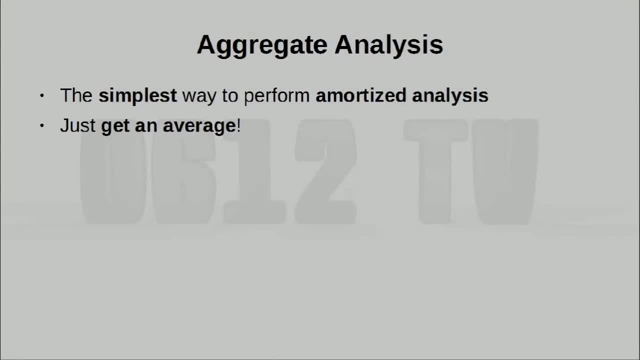 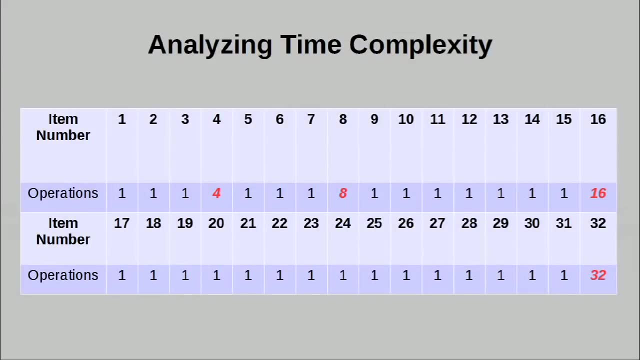 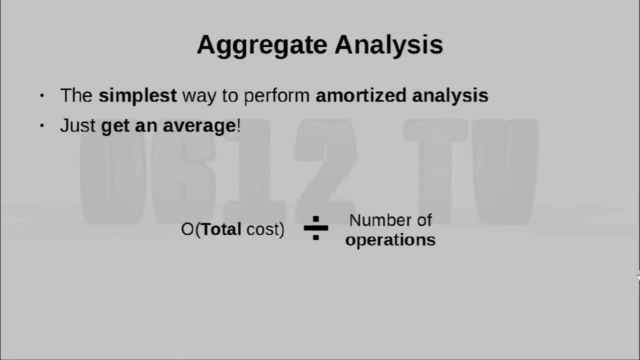 amortized analysis, and that is the aggregate method. Really, the aggregate method is just an average, And that, of course, is the simplest way of actually getting a good idea of how much work is happening per step. You want to get the total cost of a set of operations and actually divide. it by how many operations are actually happening, And that is the aggregate method, And that, of course, is the simplest way of actually getting a good idea of how much work is happening per step. Basically, you want to get the total cost of a set of operations and actually divide it by how many. 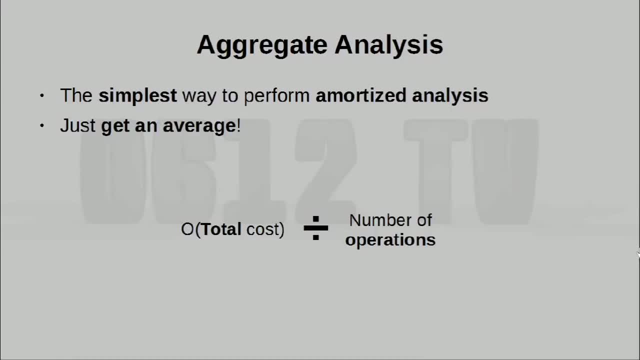 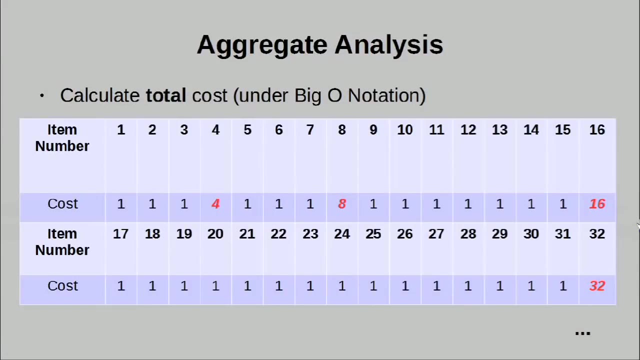 operations you've actually done in that set, And that gives you a good idea of well what the average time is required per operation. So let's actually work on both these values here. Going back to our table, we can actually calculate the total cost of however many operations. 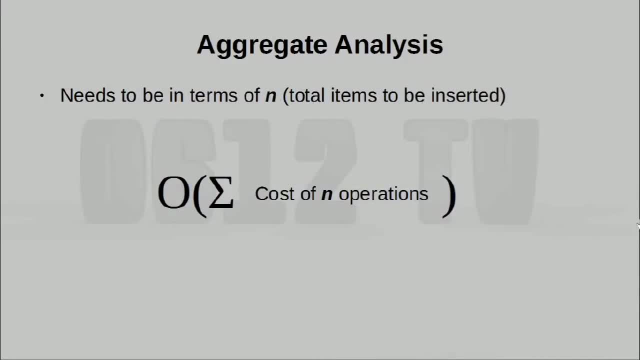 In fact, we're not going to define that, We're just going to say it in terms of n. So basically, the total cost is the sum of n operations. To make this simpler for us to understand, let's actually sort of separate this into cheap operations versus expensive operations. 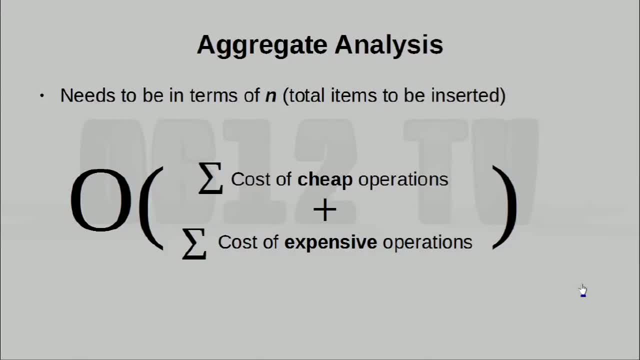 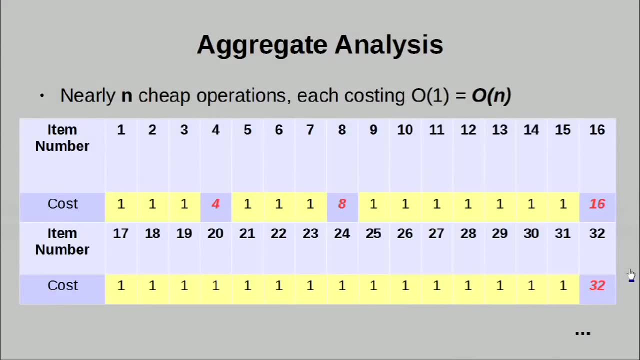 Cheap operations, of course, being those insertions that don't actually require array expansion, And expensive operations are those that do. The cheap operations are easy- They're nearly n of those if we insert n items, And since each one of these items are O1 operations, 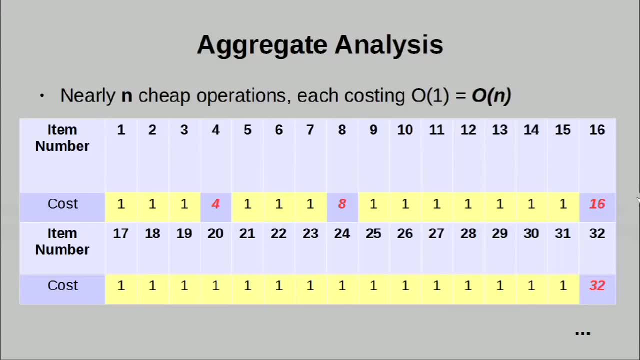 we can say that in total, the cheap operations add up to O1. It's a little bit more challenging to actually consider the expensive operations. So let's work through this together. What we're going to do is we're going to actually pretend that we started. 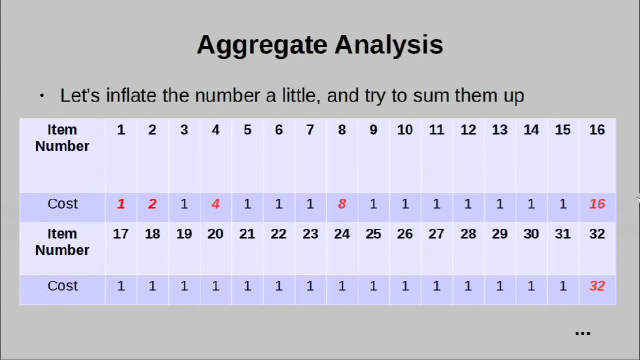 off with an array of size- 1, and we're actually triggering expansions from that. So yeah, we've actually inflated the number a little bit here, And what you of course notice is that these are just powers of 2.. 1,, 2,, 4,, 8,, 16,, 32, and so on. Now, what do we get when we try to sum all these? 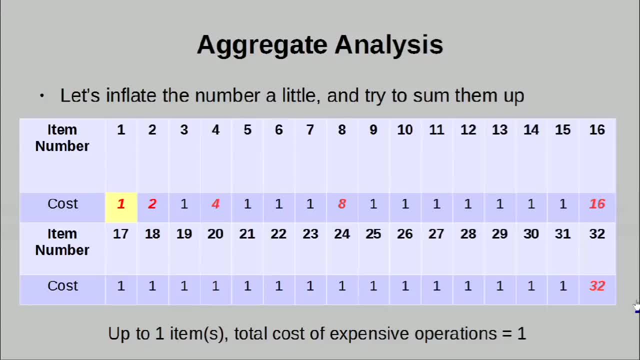 up. When we've inserted 1 item, the total cost of the expensive operations is 1.. When there are 2 items, the cost is now 3.. As we move on, we are actually piling up this number And this actually. 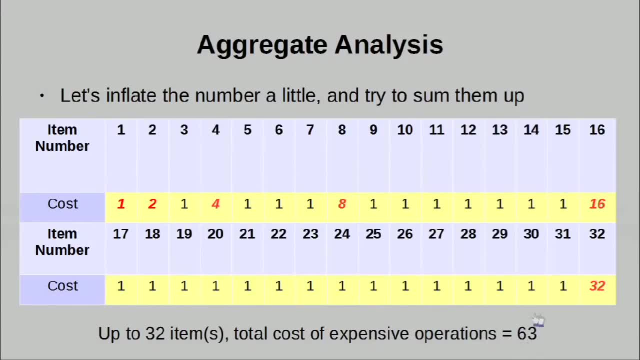 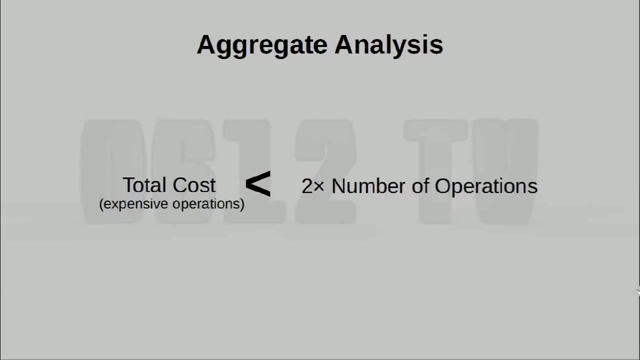 shows us a very interesting pattern. This number is approximately double of this number. In other words, the cost is actually approximately double of the number of items there are. So yeah, we could. the total cost of the expensive operations is just slightly less than 2 times the number of. 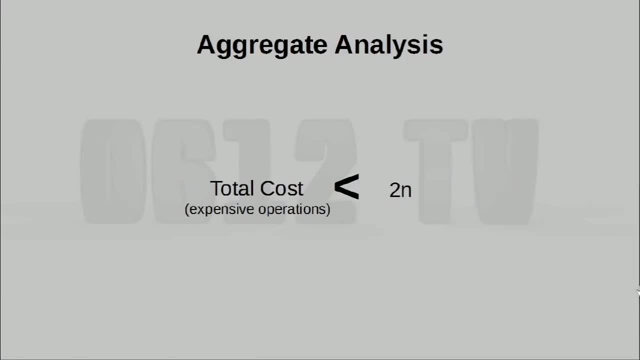 operations there have been. In other words, it's slightly less than 2n And under the big O notation it is simply o? n. Going back to our computation for the total cost. we just have to add both of these things together. At the end of the day, this, of course, simply gives us o? n. We know that we. 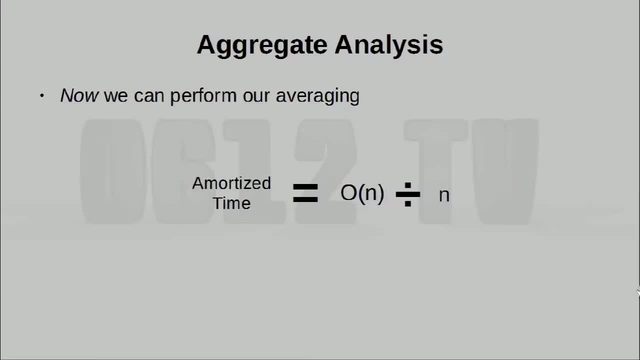 are basically performing o? n worth of work by doing n insertions. Doing our averaging, we get o? n And therefore, using the aggregate method, we now know that the amortized time of doing operations on this data structure is simply o n. This, of course, fits the intuition we've. 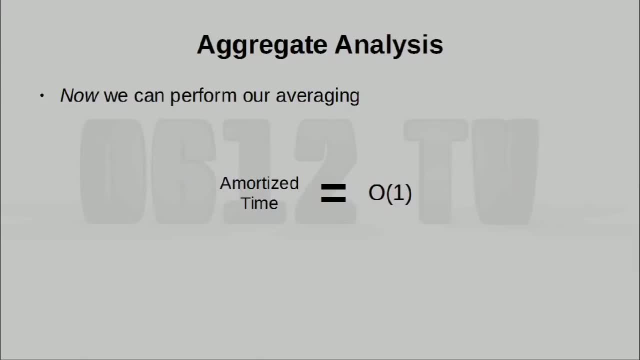 seen earlier. As we've mentioned, the work becomes twice as difficult but comes half as often, And we sort of concluded that intuitively it's going to be constant time And aggregate analysis has actually proven that to us. So aggregate analysis is one method of doing operations on. 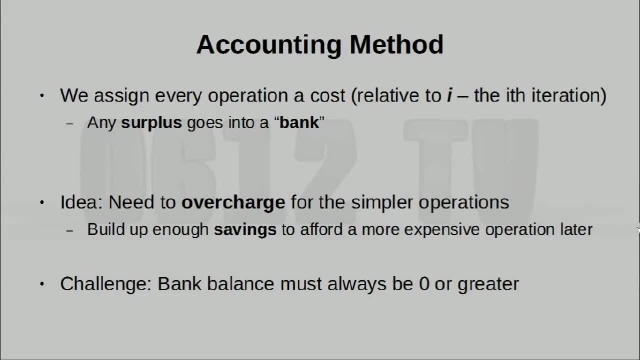 this data structure And the second method. let's now take a look at another method called the accounting method. This method takes a slightly different approach to the problem. Essentially, instead of looking at things in general, we want to jump in to look at every single operation. 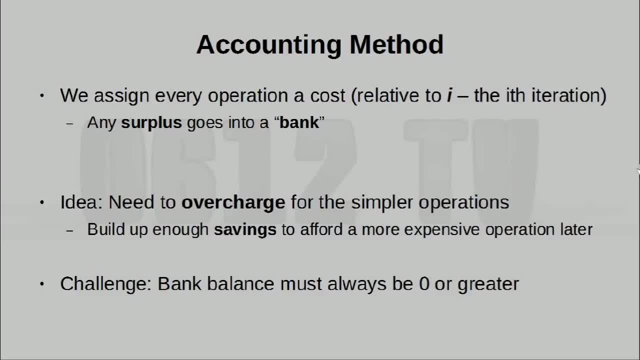 In fact, we assign every operation a cost. Normally, to go along with the accounting theme, we'll actually express the cost in dollars. If you have any surplus, it goes into a bank. The reason why we are doing this is that 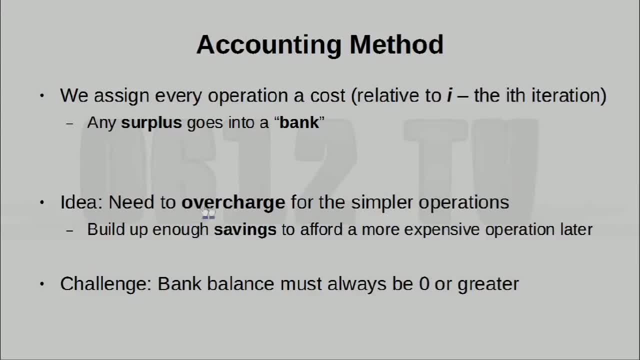 well, when we're doing simpler operations, we are actually overcharging. We'll actually give a little bit more money than it's supposed to use, And the idea is we want to build up savings enough to afford a more expensive operation later And, of course, again to align ourselves. 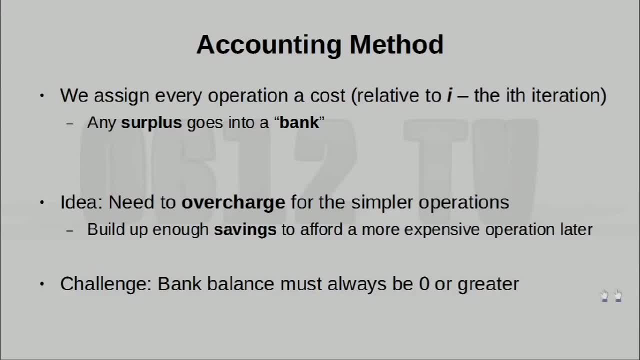 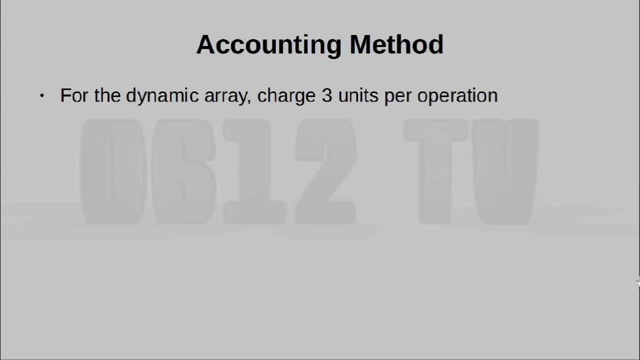 with the accounting theme. the bank balance must always be zero or greater. We don't want to be in debt. That's the whole idea. So let's actually go back to our dynamic array. The solution for the dynamic array is to go back to the dynamic array, And we're going to go back to the dynamic array. 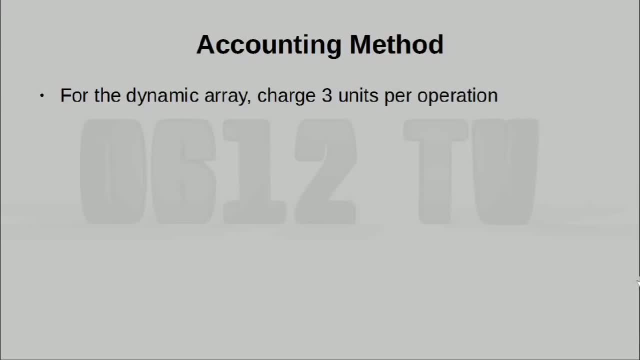 The dynamic array is to actually charge three units, or three dollars per operation. So we're going to visualize it like this: We're going to start off with a bank of zero dollars. Every time we insert an item, we're going to charge three units. Now one unit is used. 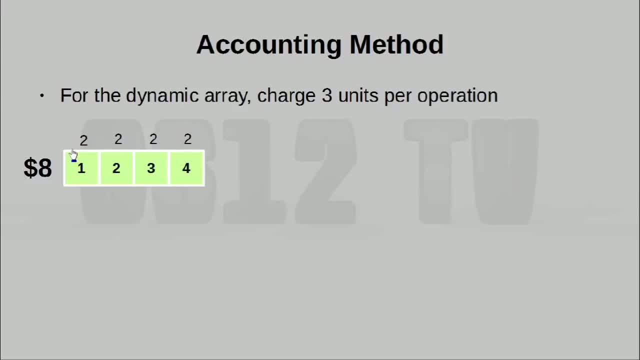 immediately for the insertion. So we have two units of surplus sitting around. So, yeah, we now have some healthy savings, But unfortunately the array is now full and we have to perform an expansion. All we have to do is to actually use up the money we have saved up to actually move the items to the new array. 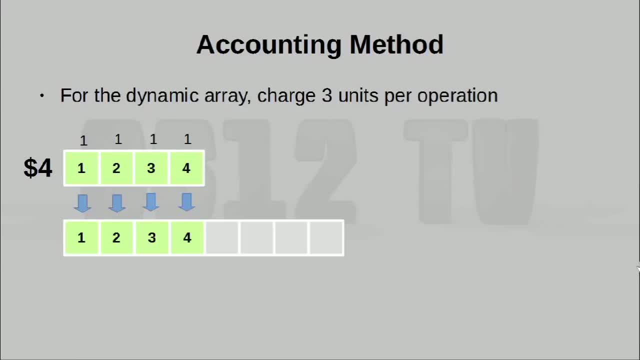 So in fact, the expansion step costs nothing. We have not assigned any money to this, because we just have to tap upon our savings. So, yeah, that's the existing state. We actually still have a dollar left for these first four items, but I want you to sort of pretend they. 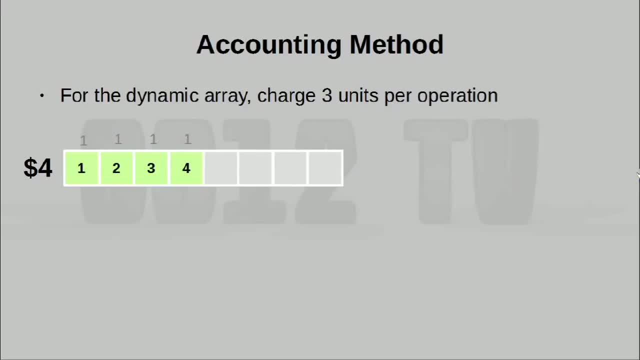 don't exist. This surplus money that's sitting here never gets used again. This is sort of an outlier, but it's worth it. So let's go back to our dynamic array, and we're going to go back to our outlier for the first four items. As we continue to add items, you'll realize that this no longer 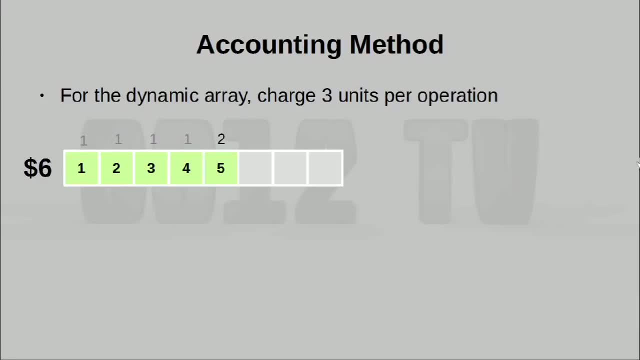 happens. Let's just continue seeing this in action. As we insert more items, we are, of course, building up our bank once again until, well, the array gets full. This is where the interesting part happens: When we create our new array, of course, items number. 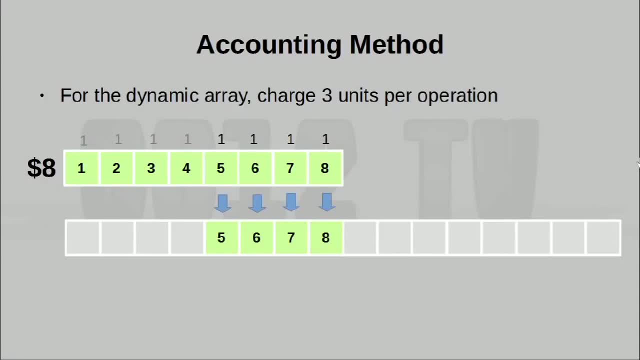 five through to eight have the savings to actually transfer themselves. What's even more cool is that we each still have a dollar left, And what this means is we can actually use the surplus we have left over to transfer items one through the four. I can use the leftover dollar from item five to 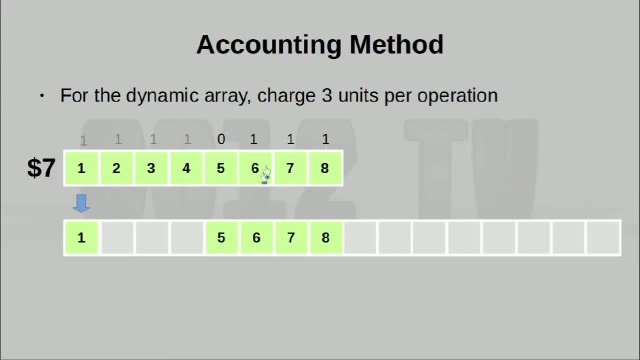 transfer item one, I can use the leftover dollar from item six to transfer item two, So on and so forth, And by actually exhausting well the remaining surplus from these four items, I complete the whole movement. So let's go back to our dynamic array and we're going to go back to our 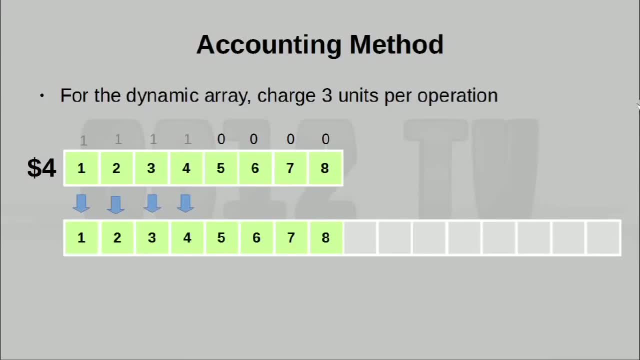 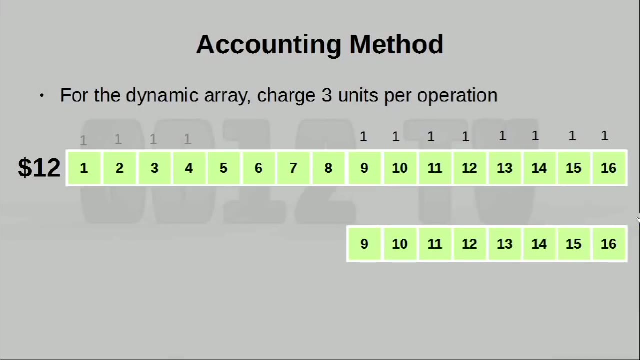 whole movement operation without incurring any extra cost. Now let's see this again: When we actually have, you know, items number nine through the 16.. Again, we'll actually have two dollars to spare for each one of these items. When we actually perform an array expansion, we can, of course, 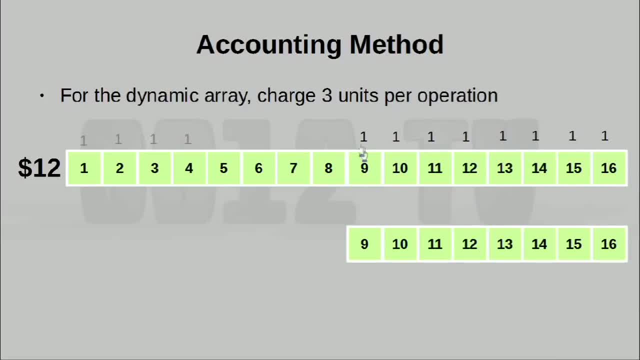 afford moving well the items themselves, But we also have enough money to move the items that no longer have any cost associated with them. This brings our bank balance back down And, in fact, if this goes on, no matter how large the 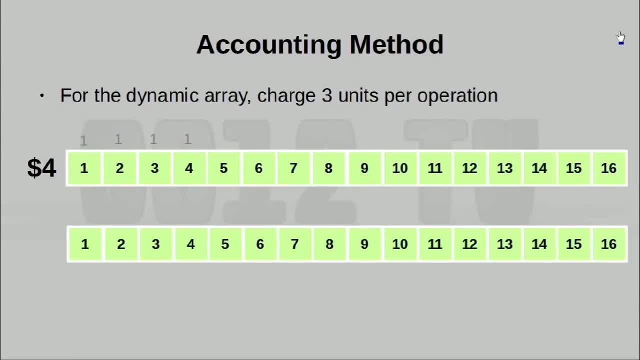 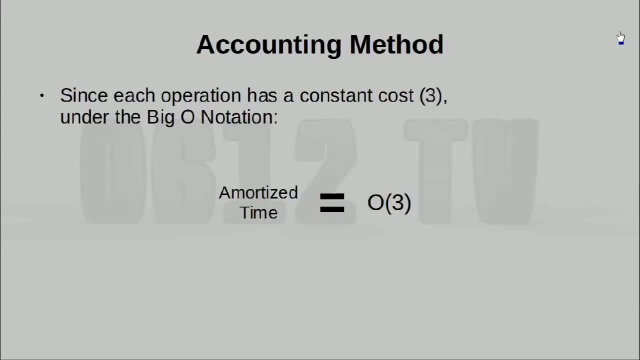 array is. this logic will continue to hold As long as each operation is actually charged three units or three dollars. we will be able to sustain this continuously, no matter how big the array actually gets, Since we now know that every operation has a constant cost of three, the amortized time. 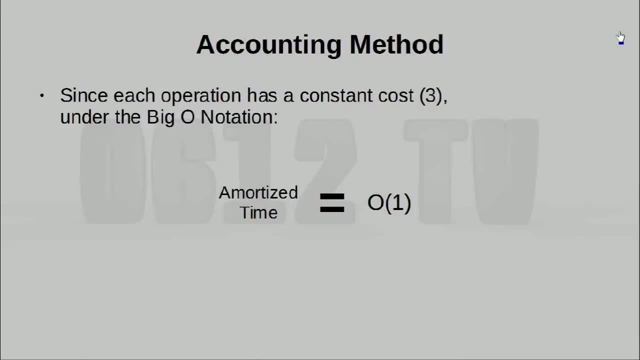 resolves itself to O one or constant time per operation. Now let's go back to our dynamic operation and see how this works. Well, let's go back to our bank balance and see how this works. Well, let's go back to our bank balance and see how this works. Well, let's go back to our bank balance. 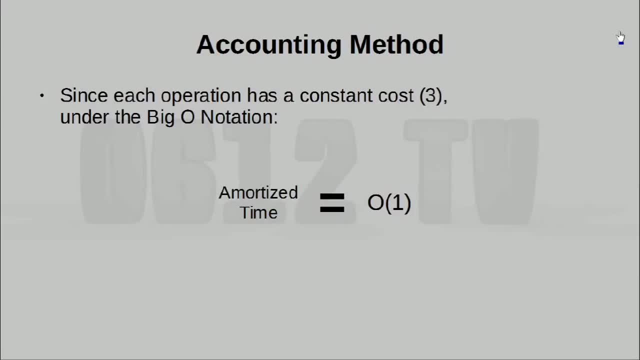 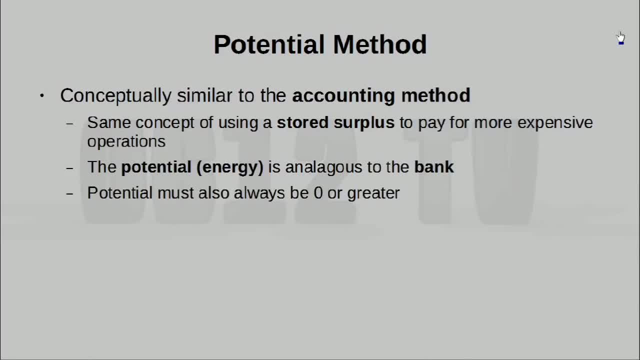 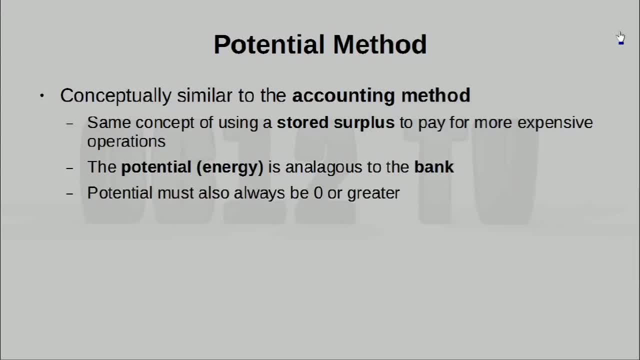 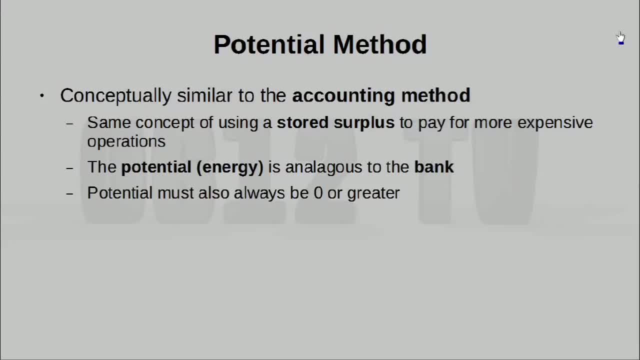 method. For each operation we want to give a little bit more. This results in a stored surplus, and this surplus can then be used to pay for the more expensive operations later on. The difference is this method is more like physics and we think of things as stored potentials. that is sort of 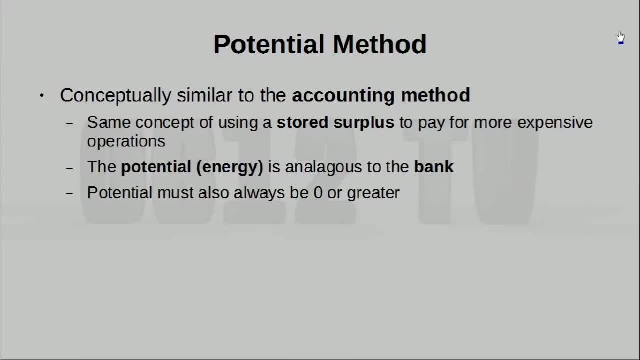 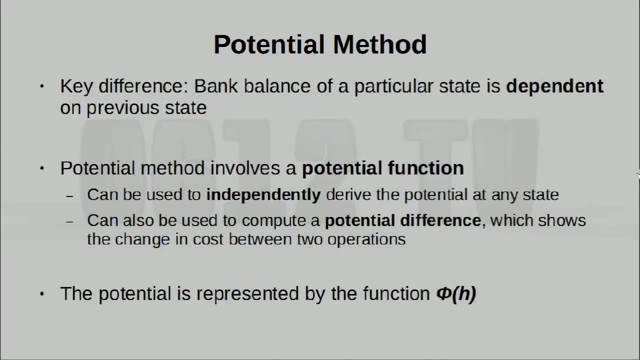 analogous to the bank in the accounting method, We are also bounded by this same limitation, and that is, we should never actually end up with a negative potential. The key difference between this method and the accounting method is that the bank balance is no longer speed dependent For the accounting. 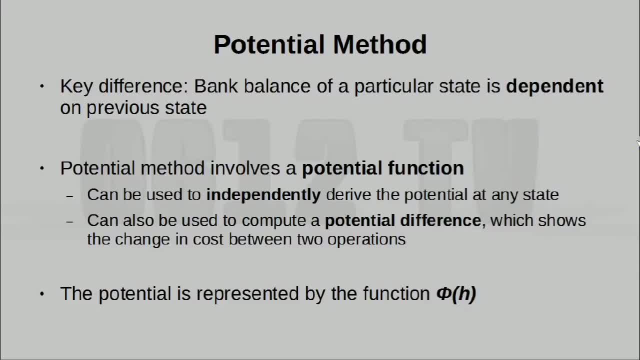 method to know how much money is left in a bank at any point, we'll actually have to start from the very beginning and work our way towards that particular point. The potential method actually makes use of a function, in other words a little equation, and we can actually use that to derive. 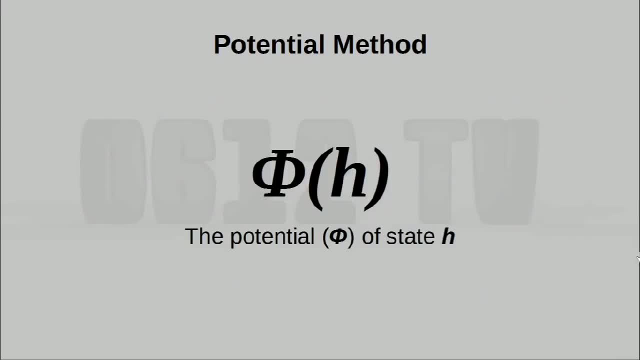 the potential of any state. Let's see how this works. Essentially, we're using the symbol phi to represent the potential of state h, So h actually refers to a particular state in a data structure. So, of course, the difficult part is to actually find a potential function that can represent, you know, the amount. 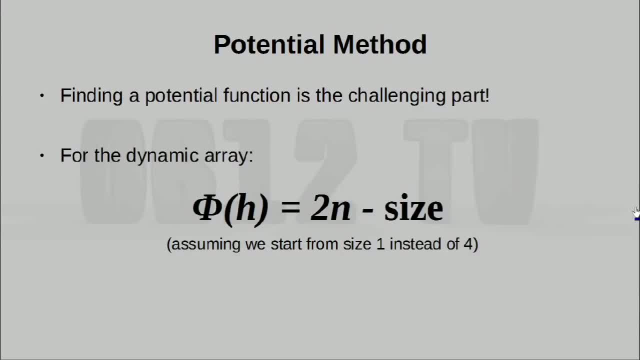 of potential at any state. In the case of the dynamic array, this is the actual function, n is the number of items we have inserted so far and size refers to the actual size of the array, Including the actual elements in the array that haven't been filled yet Now. in all the examples, 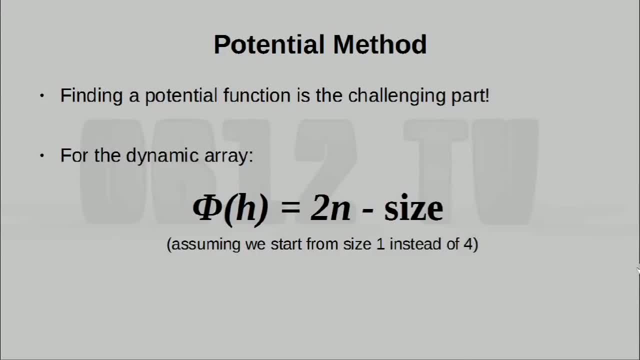 up to this point, we've actually started with an array of size 4, but what we're going to do is this actually assumes we start from size 1 instead. So, yeah, let's actually, you know, work with things this way instead of starting from size 4.. It's not going to be hugely different When there 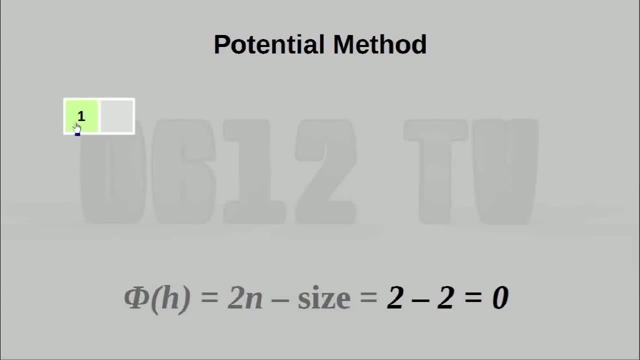 is one item, we will have to actually expand to size 2.. Therefore, our potential of 2 times n minus gives us 0.. That's great, That's fine, That's not a problem. Again, when we have two items. 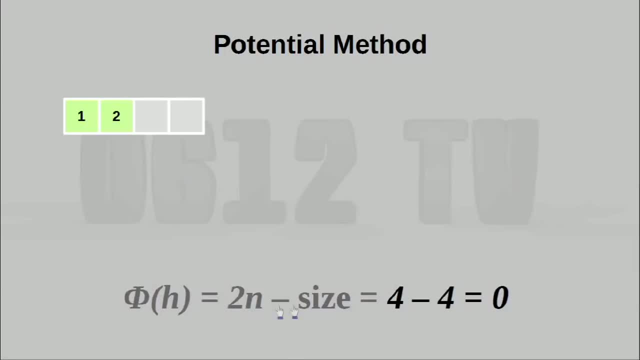 the array would have resized itself to size 4.. Our formula again gives us 0.. When we have three items, we do actually have a little bit of spare potential. However, when we add yet another item, well, the size has increased and we get a potential of 0 again. So yeah, by just taking 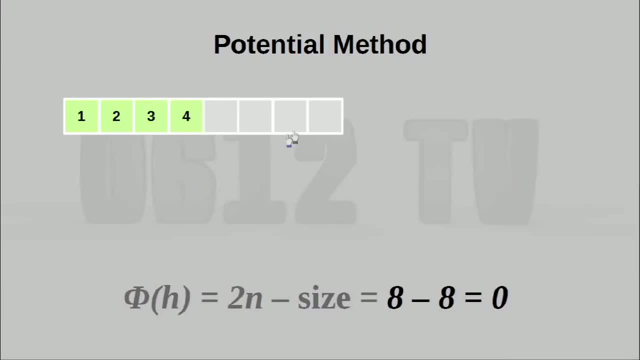 double the number of items in the array minus the actual size of the array, we'll get a potential of 0 and a potential that is 0 or greater at all times, As mentioned. of course, the cool thing about this is that we can actually check the potential at any point, For example, if we're 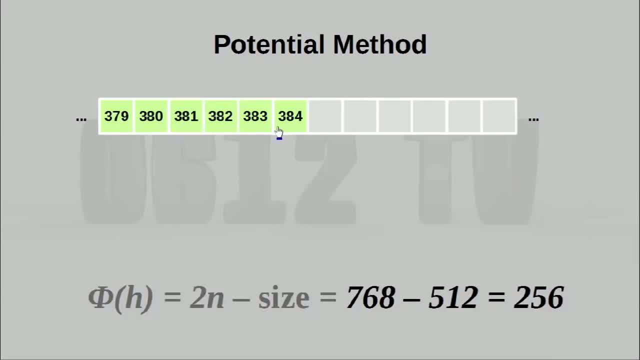 now at item number 384,. well, no problem, We can simply insert that into this formula: 2 times 384 minus the size, which, of course, we know that the closest larger power of 2 is 512.. This tells us there is this much potential left. 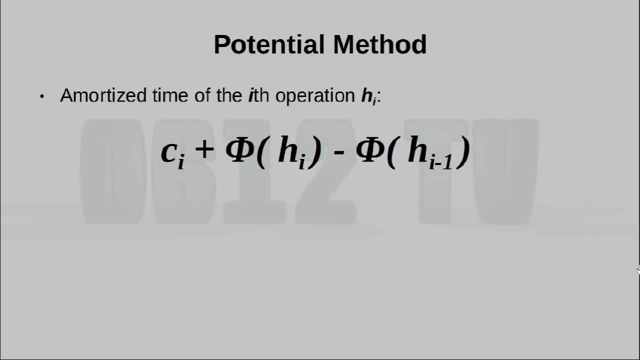 Now, if we actually calculate the amortized time of the ith operation, in other words h i, we'll actually do something that looks like this: Now, I know this is a little bit complicated, but essentially what you have here is a potential difference, The potential of the current step. 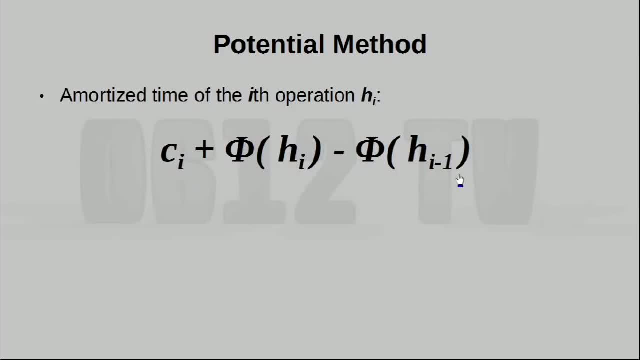 minus the potential of the previous step. That is of course how we get a difference between any two values. really, The amortized time of operation. i is to actually add the cost of that operation to that potential difference. So if we add the cost of that operation to that potential, 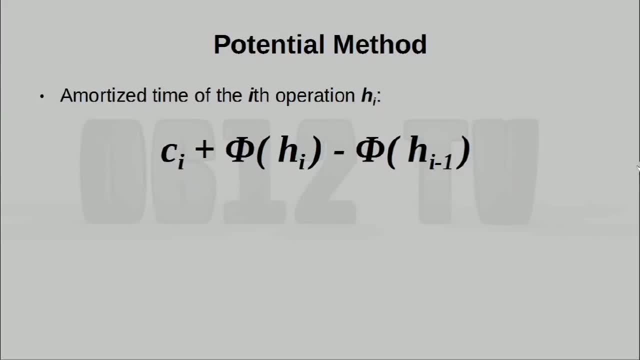 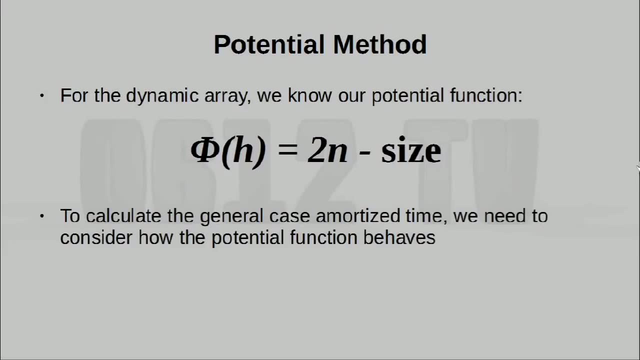 difference. I know this is a little confusing, but once we put it in action it will be okay. Of course, we know that our potential function is 2n minus size, So of course we can simply use this to calculate the general case: amortized time. Now here's the deal. We need to know that. 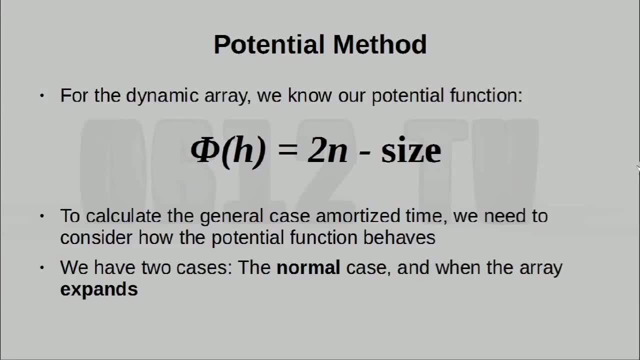 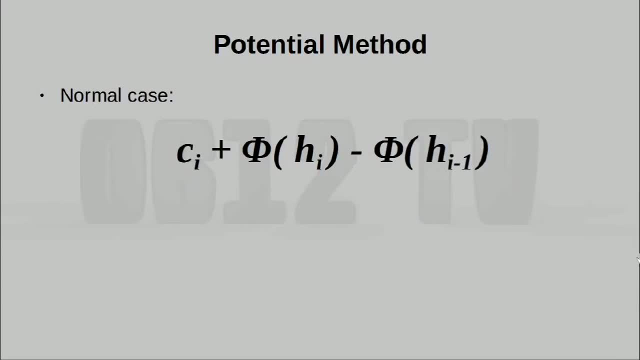 our potential function actually behaves in two different ways. There is the normal case as well as the array expansion case, So what we're going to do is we're going to look at them separately. So let's assume that we're talking about a potential function that is 2n minus size. 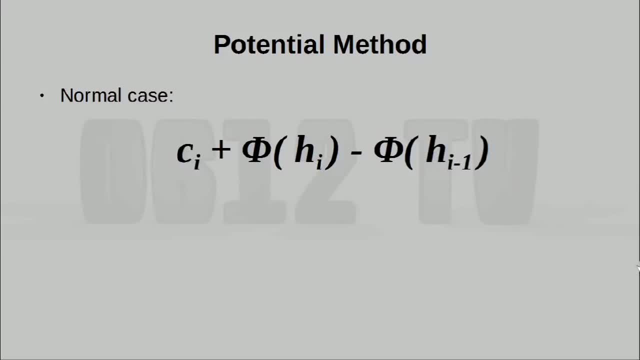 We're talking about a normal case here: no array expansion. Let's actually insert all these numbers and see what it works out to. So we start by actually substituting the potential function of the current step and the potential function of the previous step. Don't be too intimidated by 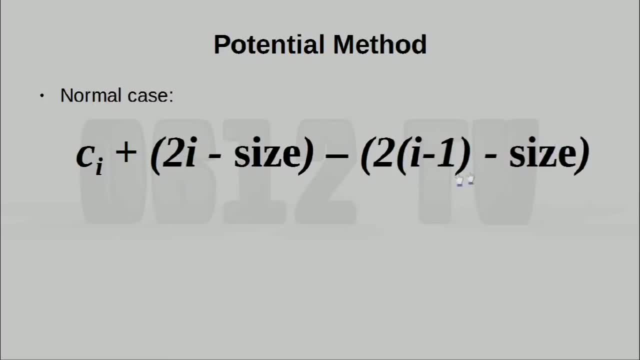 this. This just comes from the potential function, And we've of course substituted i minus 1 for the previous step. Now, since this is a normal case, the cost of this operation is simply 1.. We've just inserted one item, So no big deal. Let's do a little bit of algebra. Let's go ahead. 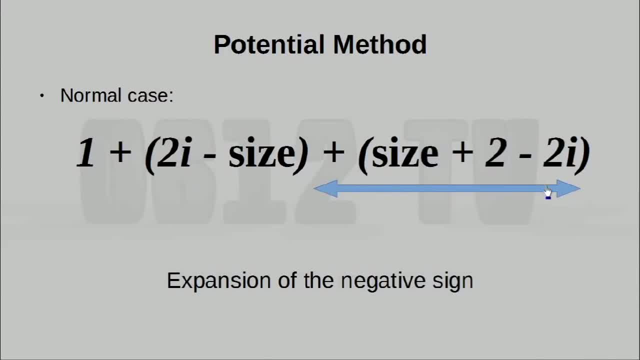 and expand this stuff inside here, Multiply in the negative sign, Get rid of all the brackets, And what we notice is that nearly everything cancels out. The size cancels out, since it's the same value. 2i cancels out, And what we're left with is 1 plus 2 or 3.. So this in fact, 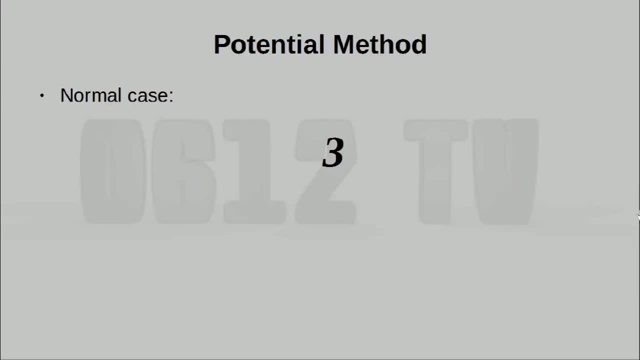 is giving us the exact same result as when we actually did the same thing. So we're going to actually use the accounting method. Of course, we're not quite done yet. This is the normal case. Let's actually look at the expansion case. The cost is not just 1.. We're actually going to have 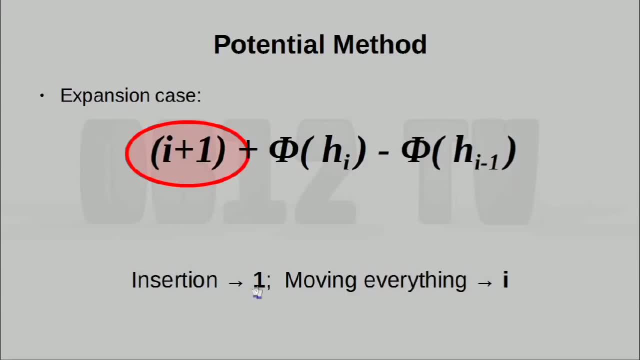 to do i plus 1 operations, because insertion requires one operation and moving everything requires i operations. since there were i items in the actual array, Substituting the actual potential function is a little bit tricky since, of course, the value of size is now. 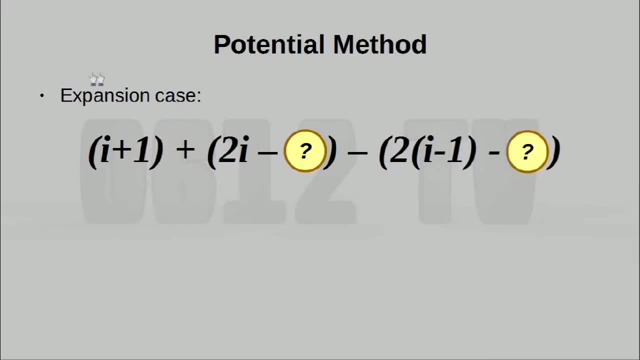 different. So let's go ahead and do a little bit of algebra. Let's go ahead and do a little bit of algebra. Let's go ahead and do a little bit of algebra. Let's look at the same thing. Luckily, since we know we are at the array expansion case, we know that i is essentially 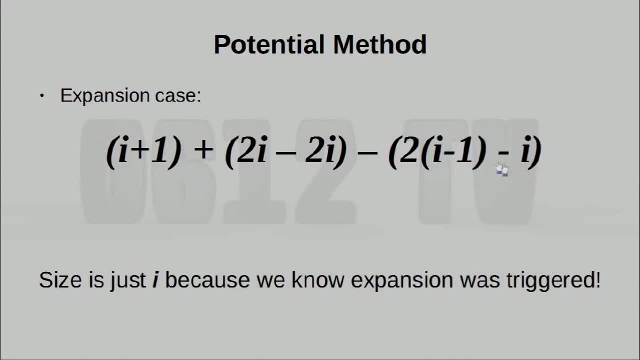 the size. Before we perform the expansion, the size of the array is i. After we perform the expansion, the size of the array is 2i. So, yeah, all that's left to do, since everything here is in terms of i and constants, well, we're just going to get rid of all the brackets, put everything. 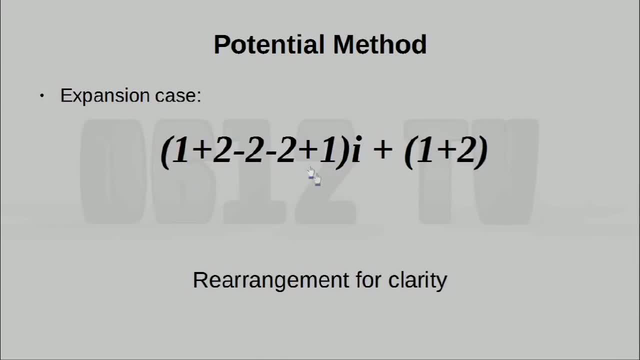 together and guess what? All the coefficients are going to be the same. So we're just going to I cancel each other out. we end up again with just 3.. So yeah, since there are only 2 cases- the expansion case and the non-expansion case- and they both give us 3 operations in amortized 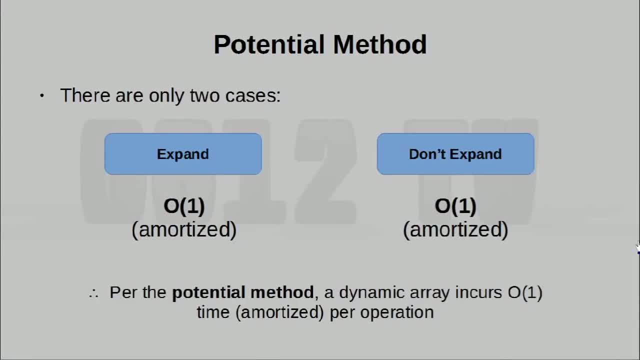 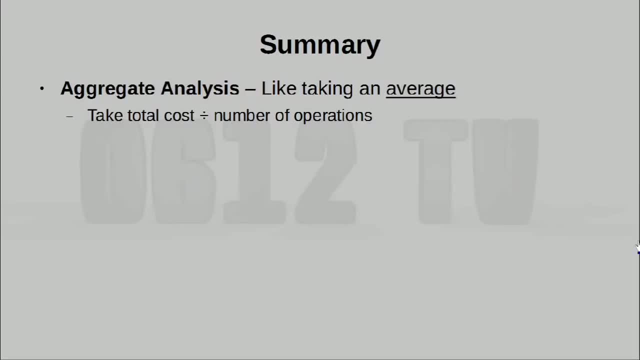 time? well, it's 01.. We can just conclude that, per the potential method, any operation incurs an 01 amortized time. So, yeah, well, we've actually gone through a lot of content today, so let's very quickly summarize. First of all, we have an aggregate method which 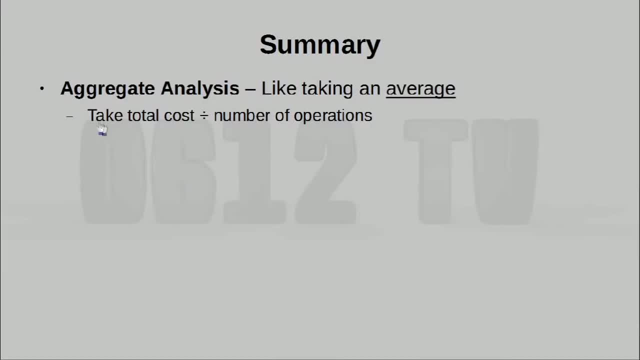 is like taking an average. Simply put, this method is taking a total cost divided by the number of operations that ended up incurring this cost. So yeah, in fact this is one of the simpler ways. If you actually want to move on to more complex ways you can use. 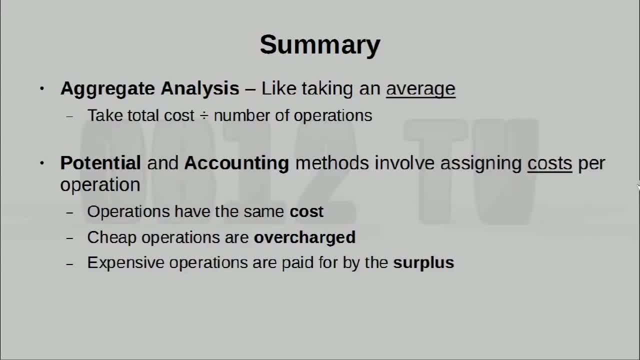 the potential or accounting methods. Conceptually they're the same. we want to assign a cost to each operation. Cheaper operations are overcharged, which gives us a surplus, and expensive operations are paid for using that surplus. The difference between the accounting and potential methods. 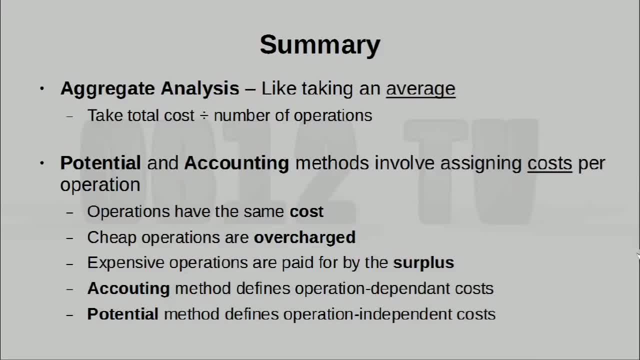 is that the accounting method is actually operation-dependent, whereas the potential method actually defines a formula that tells you the potential at any point of time. So you can think of this as the slightly more rigorous way of doing the same thing, while we end up with the same result. 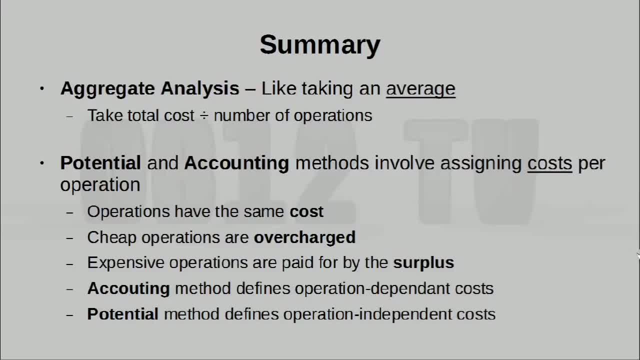 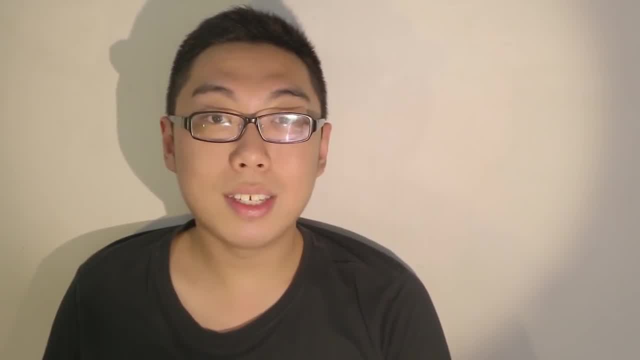 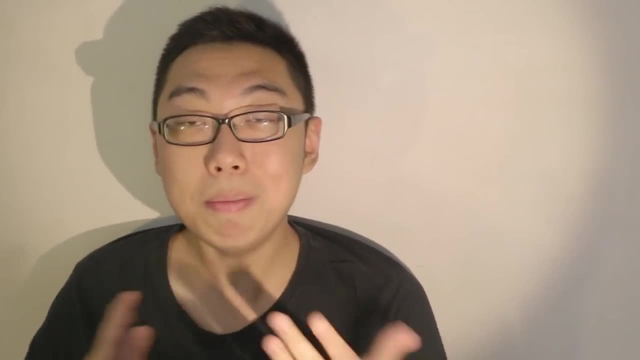 This method is more robust because it is operation-independent. As a drawback, it is, of course, more mathematical. So there you go. that was amortized analysis. We've just taken a look at three different ways to actually perform amortized analysis, and we applied it to the most classic example. 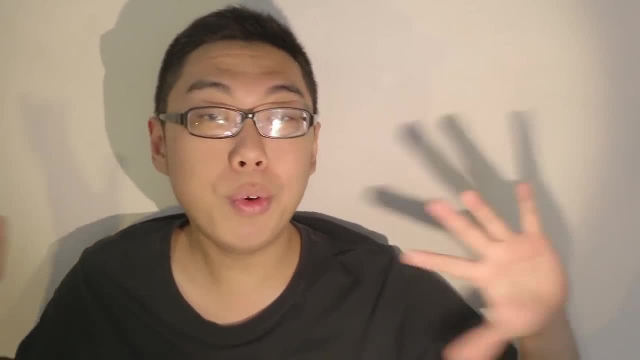 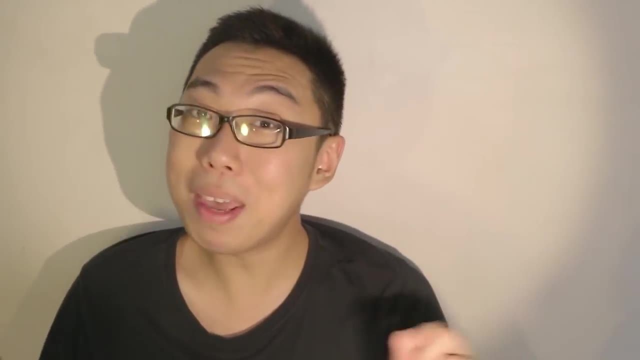 which is the dynamically resizing array. As mentioned, we've just scraped the surface today. Applying amortized analysis on real, hardcore data structures may not be the best way to do it, but it's worth taking a look. It may be a lot more difficult. there may be a lot of staring at it and just waiting. 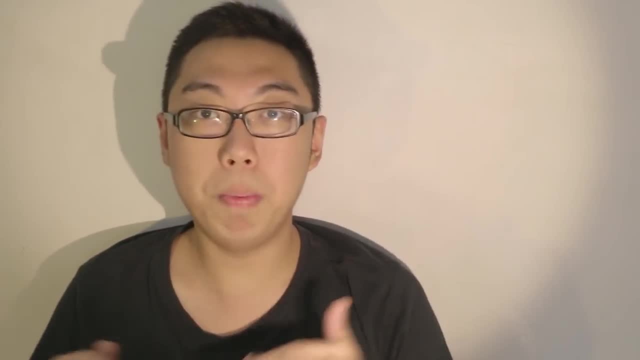 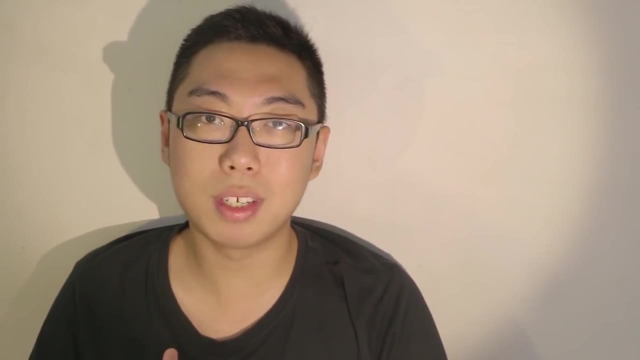 for the intuition to jump out at you, but the fundamentals remain the same And hopefully what I've done for you today is I have painted a rough picture of all these fundamentals. Anyway, that's all there is for this particular episode. I hope I've been a help. Thank you. 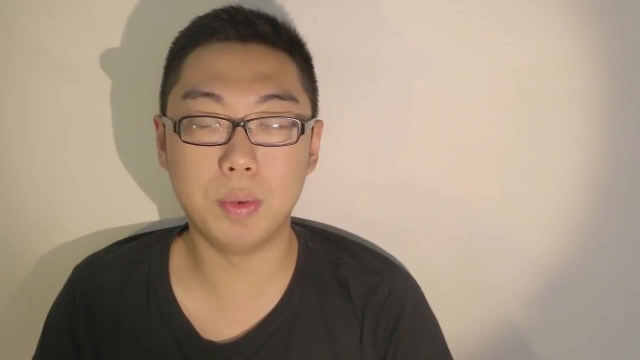 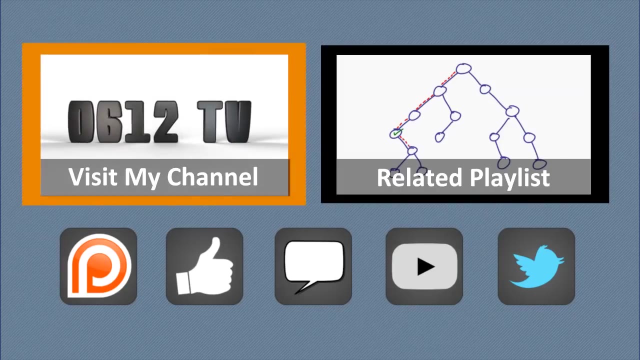 very much for watching and until next time. you're watching 0612 TV. Thanks for watching and if you liked this video, consider checking out the rest of my work on my channel. Alternatively, you may be interested in a playlist of my earlier. 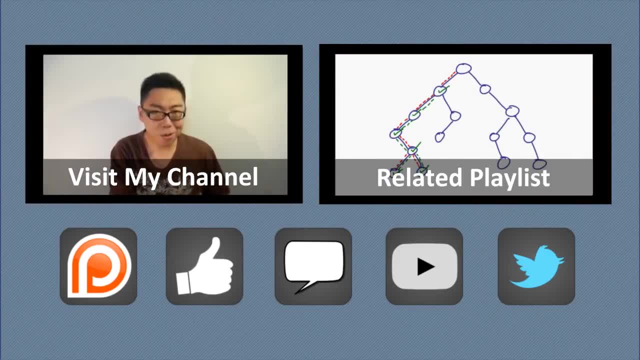 work on computing and computer science topics. If you'd like to show me some monetary support, I am on Patreon. You can find a link to my campaign in the video description. Of course, you can simply like this video or leave a comment. I'll be sure to respond as soon. 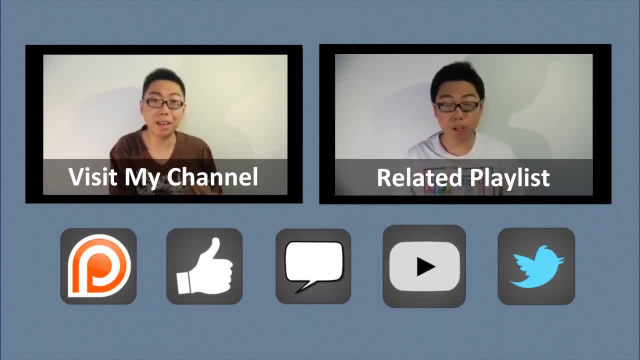 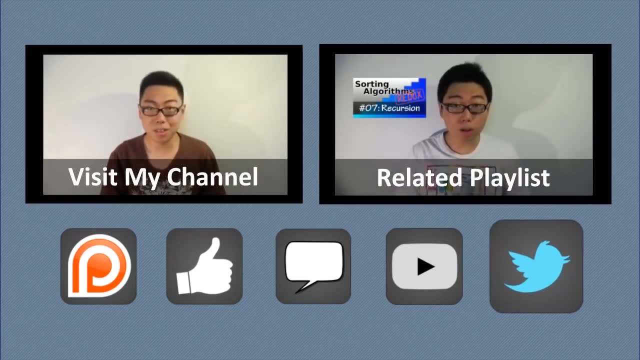 as I can. To keep in touch with my future uploads, do subscribe to this channel and, for even more updates, click the link in the description. Thanks for watching and until next time. I'll see you in the next video.